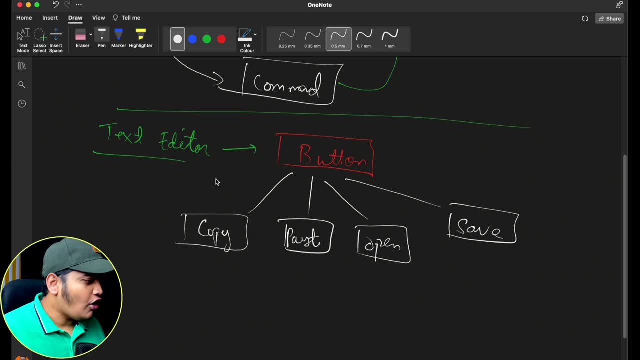 Right, Okay, So these are the different buttons that I'm creating. Okay, for all these buttons, my button class, my button interfaces are based on An object And all the different functionalities, all the different buttons will have the different business logic. Okay, copy will. 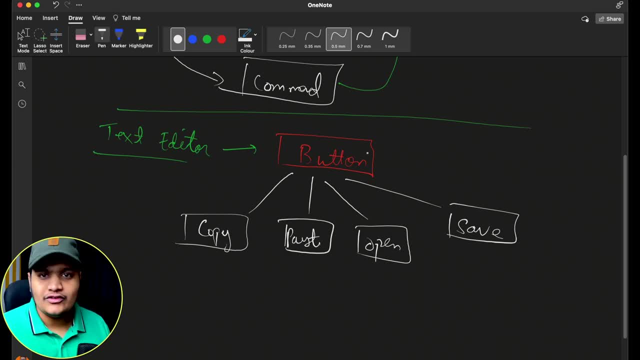 do copy paste will do paste, open, save. Similarly, all the buttons will do the different things. Okay, so that's one of the scenarios, and what it will happen is you will be creating a different subclasses to have this functionality. Okay, so you will be doing this way. Now suppose, 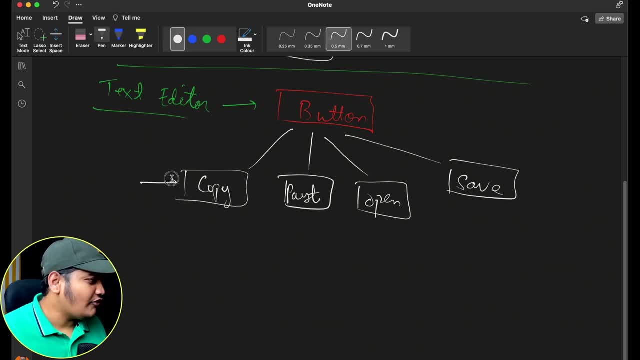 one more situation comes: that, okay, you've created all the various methods. you could be زر. you have written the logic of copying. okay, like how to copy, like data and everything, So that business logic is written already. Okay, now there's a functionality like when: 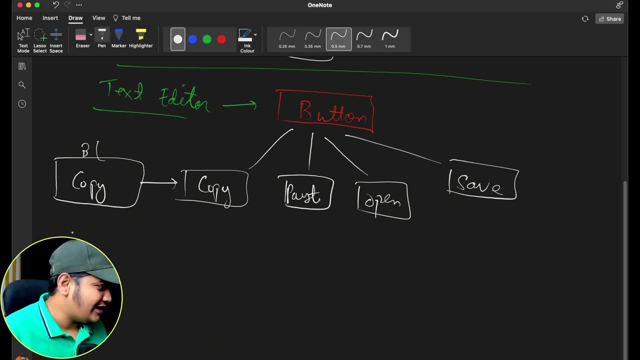 you do a copy. okay, what we can do is we do a Ctrl C as well, like copyright Ctrl C or Command C to copy. So that is also one functionality. So when you do this Ctrl C, at the same time you have to invoke the same business logic that you have written for the 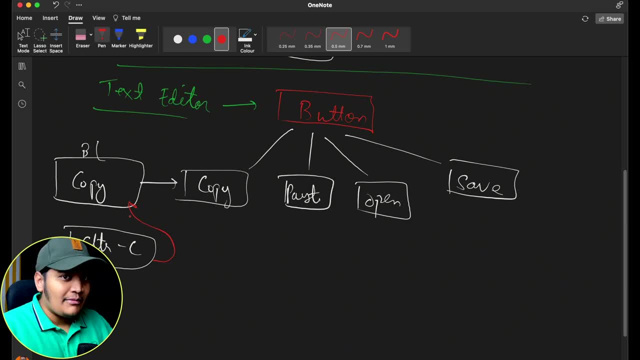 copy. Okay, so you can see that your business logic, your command execution, is same for multiple things. now, right, Not just button, you also have a shortcut that does the same thing. okay, that does the same. copy paste upon whatever it is. okay. So now you have. 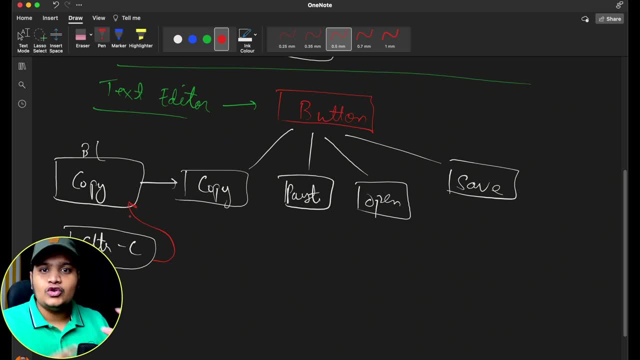 two different types of command that can do the same thing. Okay, one is button click, event and one is shortcut. Okay, so that way, that is a button click and one is a shortcut. Now, there might be multiple things can be added as well, right? So for each and everything. 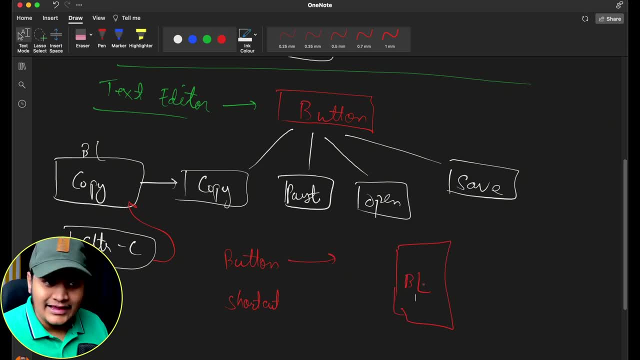 if you are doing a request to the business logic layer to do the same thing, like to, when you click a button, when it's a copy button, do this copy button operation. when the shortcut is Command C or Ctrl C, do the copy operation. you can see that you will. 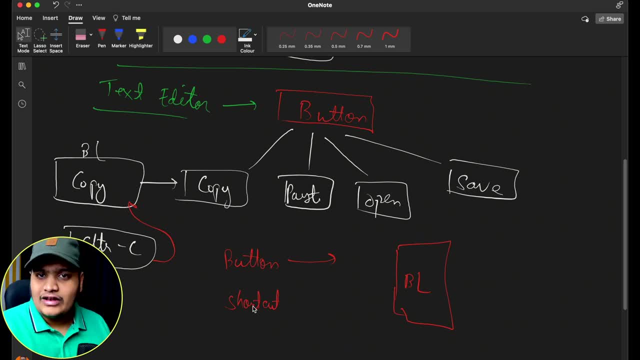 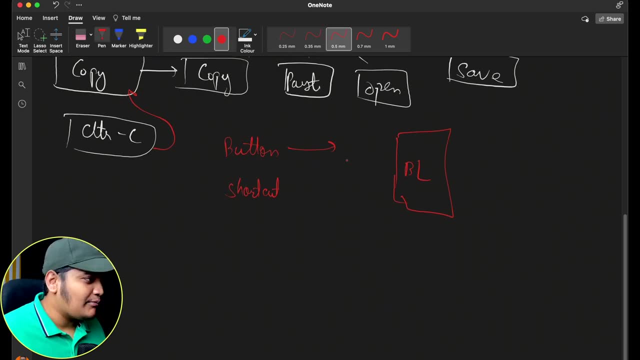 have a lot of duplication of the code and a lot of things will happen, and maintaining that code will also be difficult at that time, right? So, rather, what you can do is for any type of request that you receive, right, any type of request that you receive, what you. 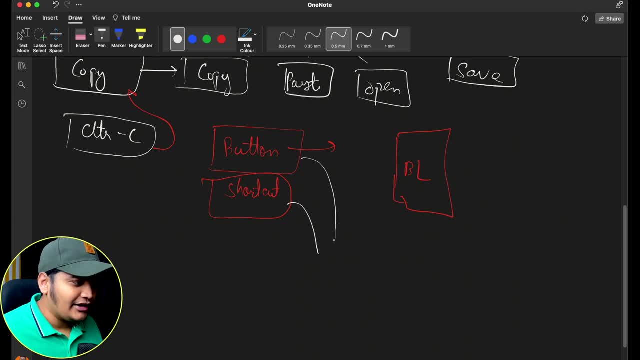 will do is that all the request can be converted into a command. Okay, And this command can be executed by your business layer. Okay, your business layer will get that command and that command will be executed. So whenever I click a copy button. okay, it. 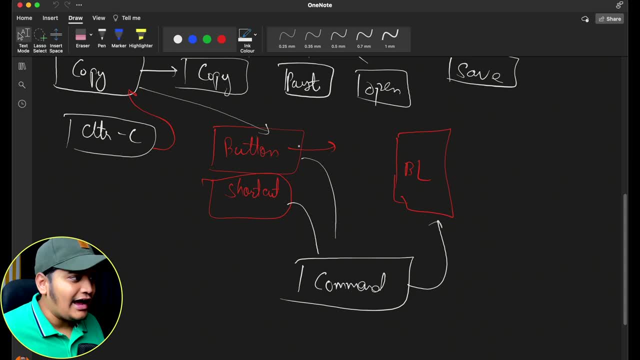 will can. it will take that request, will take the input data and it will create a copy command. Okay, I will create this command as a base interface. Okay, and multiple interface and multiples concrete classes can be implemented by this command. So I'll create a command. 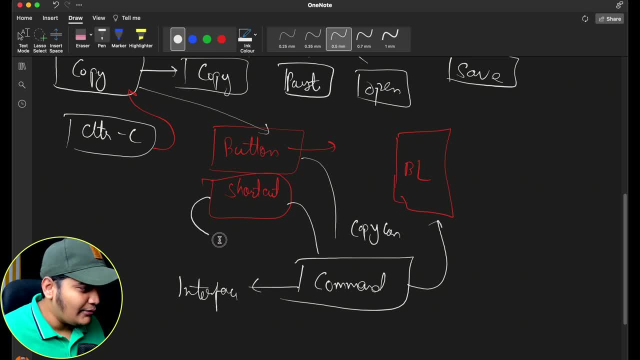 Okay, this command is a copy command. when I click Ctrl C, at that time also, I'll create the same command. Okay, And this copy command will be passed along to the receiver and that receiver will perform that operation over here. So that's the basic idea about converting any requests directly. 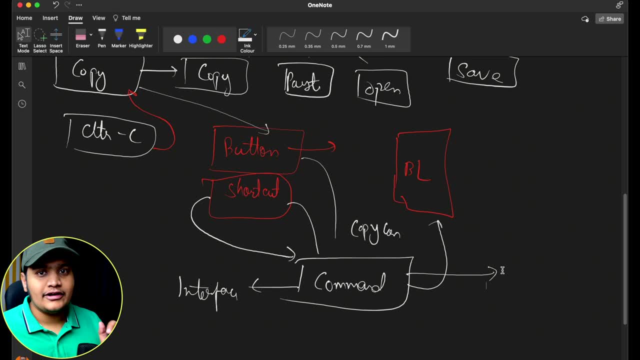 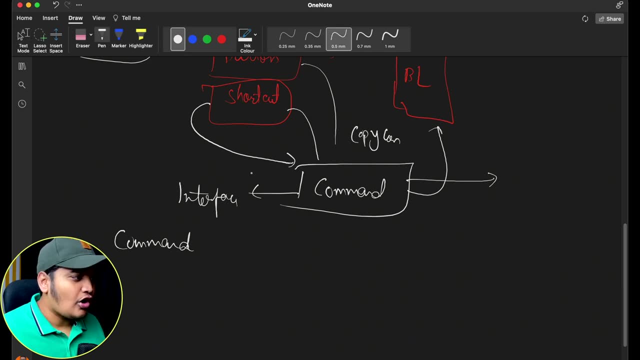 been executed to a command, and that command can be executed. Okay, so there are different components to it, So one of the component is command itself. Okay, so you can see that these are the all the commands that we created, right, So any command can be executed. So. 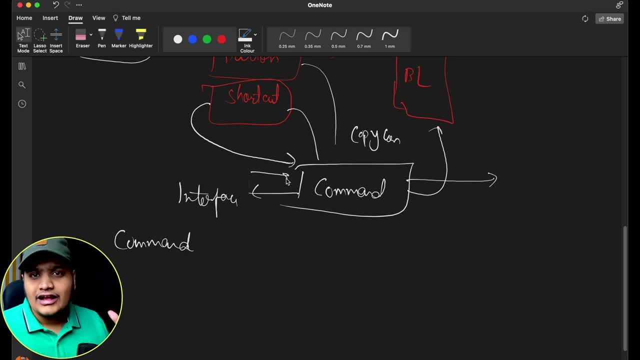 that's a basic command. you will create an interface for it And different commands can be implemented. concrete classes can be created to have that command executed. with that command, there is a receiver as well. okay, there is one component called receiver. so what receiver is receiver? 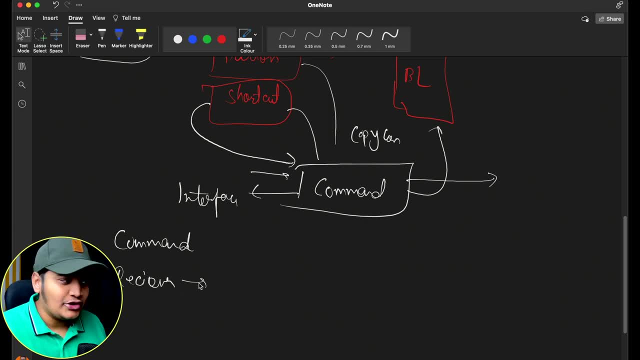 is actually a particular component that will be executed. so suppose i want a command that is the open file. okay, so this is the command and receiver would be file itself. like this, file will be open, file will be saved, file will be copied. so all that operation you can. 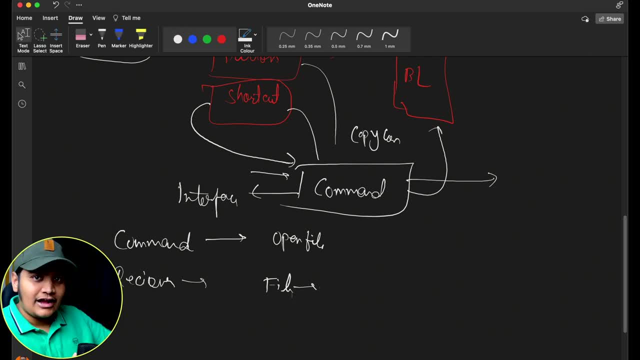 see will be the part of receiver. that receiver will get the command. okay, i'm a text file. okay, consider, this is a text file. this text file will receive a command to open. so that's a receiver. and this receiver will do that operation. okay, so that's the receiver part. 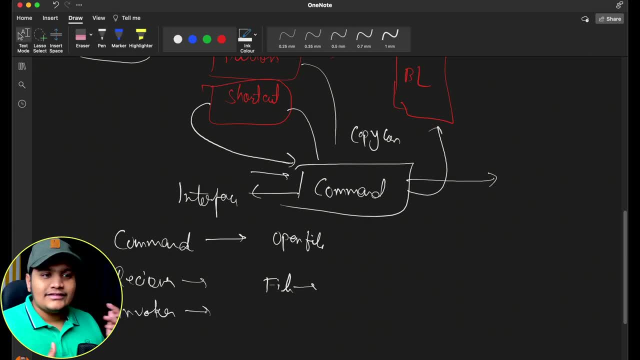 one is the invoker part. okay, this invoker will be invoking all the different requests. this invoker have the list of different commands to be executed on receiver and that particular invoker will be be executing all the commands one by one. This is very helpful when we want to do redo. 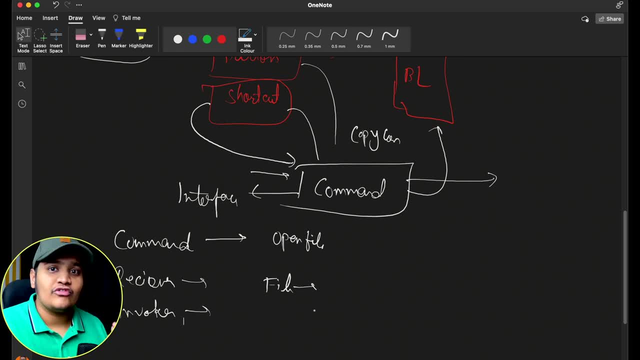 operations or undo operations. at that time this type of invoker is really helpful, right? So I will have the list of commands that are already executed on a receiver. Okay, So suppose two couple of copies were done, couple of piece were done, couple of cuts were done, 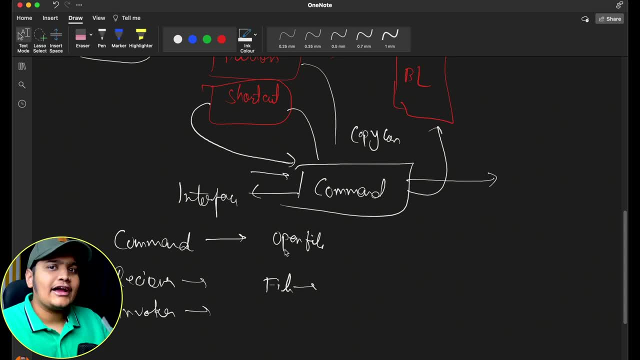 all those lists I will have And if I want to undo or redo I can do all those commands and all those commands will also have the data to it. Okay, So this way invoker will have, invoker will have the list of commands and those commands can be executed and one. 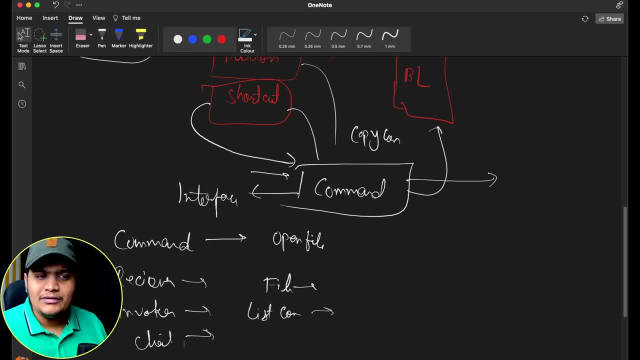 would be client right. Client will be the one which will be using the invoker to invoke all the functionalities of the command design pattern. So these are the basic components of a command design pattern And I also explained you the basic, like when we will be using this command design pattern, like when we, whenever we- 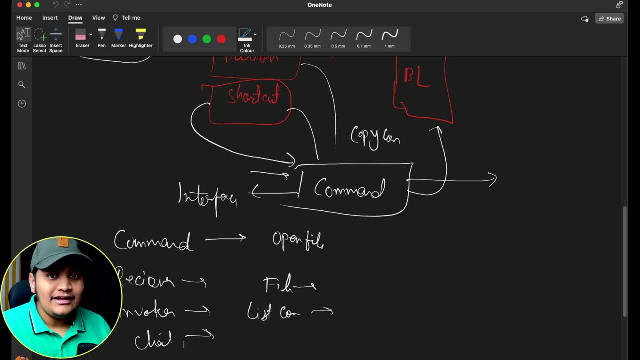 want to have the implementation by multiple places, right? Multiple things are calling the same thing. at that time, rather than duplicating the code, we can create the command out of it, And that command design pattern is called the command design pattern And that command. 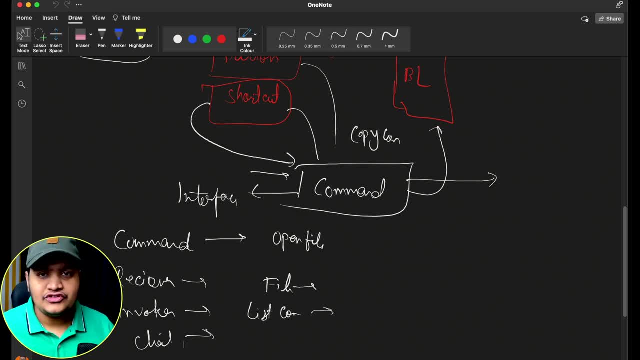 can be executed by any of the receivers. Okay, So, when this type of situation arrives, we will use the command design pattern. Okay So, one is like creating a command and one is like executing that particular command. Okay, So, that is the type of relationship. 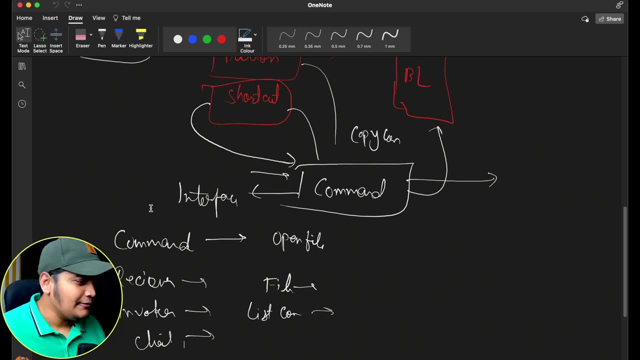 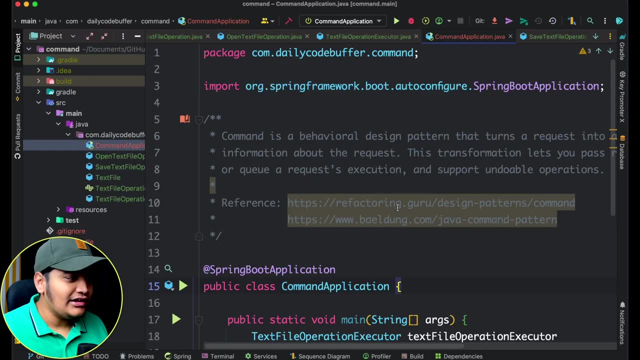 we are expecting here, Okay, So let's understand with the code here. Okay, We will be using the same example for the text file. So let me just open my IntelliJ IDEA, And here you can see that I've given you the definition as well And the references that I've used. 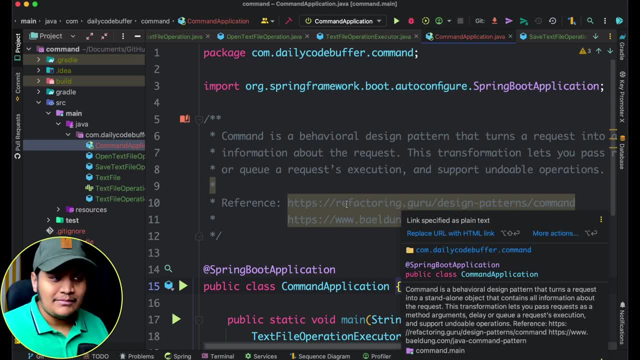 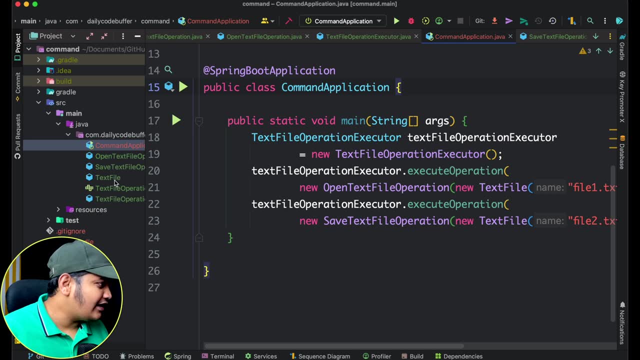 you can go to this references and you can understand more about the command design pattern and you can support the creators as well. Let's first understand about the command. Okay, So here you can see that I've created a command that is the text file operation. Okay, This is the interface I've created and 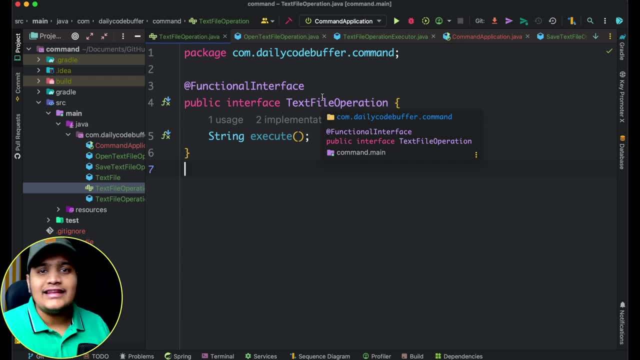 I've created as a functional interface so that this can be used as a Lambda expressions as well if we want to use Okay. So that's why this is not mandatory, but it should be interface and this interface can be implemented by implemented by the contract classes. So 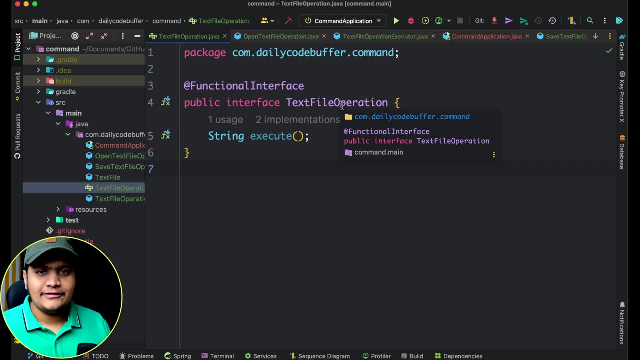 that's the text file operation. So I want to do any operation on a text file. That's the command I want to do. And this command, you can see it has a method that will be executed. Okay, To execute a particular command. So this is the interface. 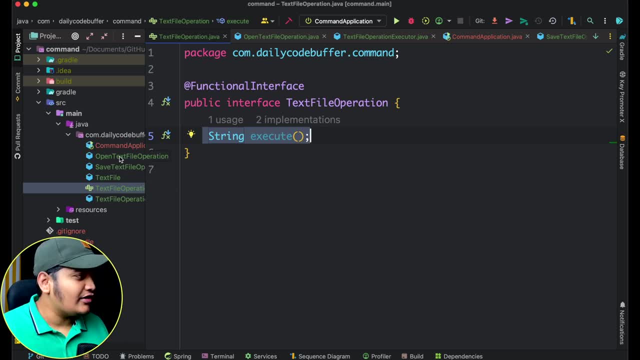 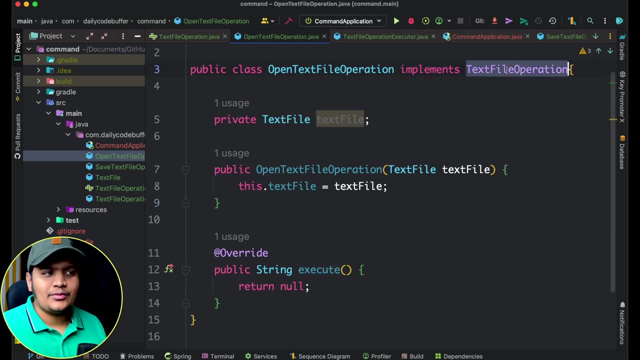 Now let's implement this interface. So this interface you can see. I have created one more operation that is open file. That's the open text file operation, which is implementing text file operation. So you can see that this is the concrete class implementing the command. 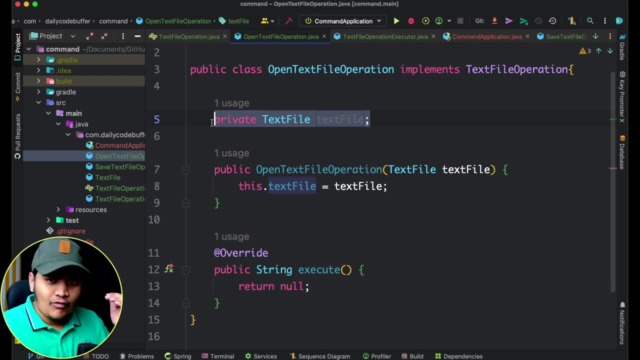 And yeah, you can see that I have the reference of the receiver. Okay, Like what is the receiver which will be going to implement or execute this command? Okay, So for my open what I want to open, I want to open a text file, So that text file is my receiver, That text. 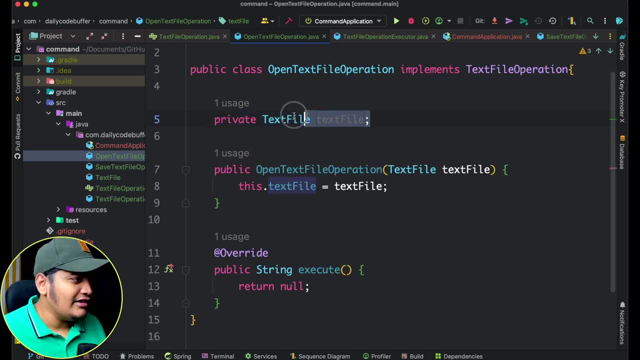 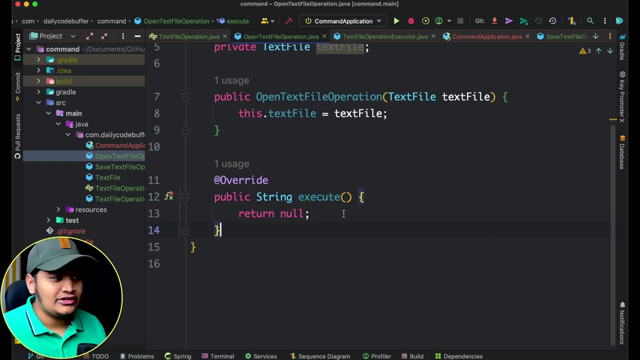 file will be executing that particular command. Okay. So that's why I've given receiver here And this is the constructor to pass the receiver here, And you can see that this is the method Okay Which is returning now. So that means I have just implemented this particular method. 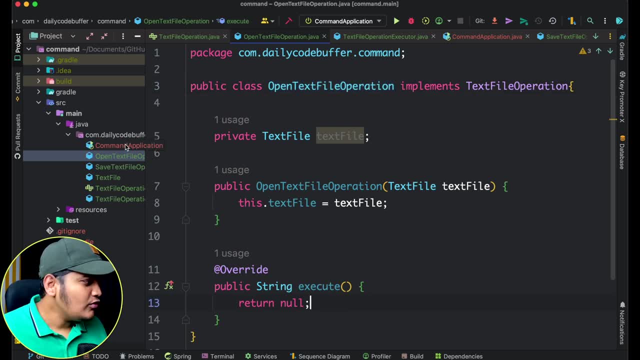 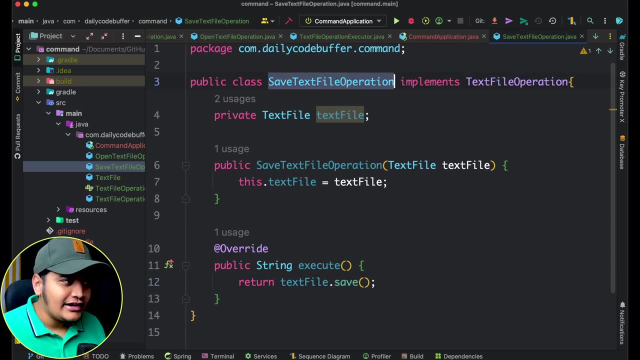 You can do any operation over here. Okay, That's fine. Now same thing over here. That is the cell text file operation which is implementing text file operation. That's the same thing. This is the concrete class which is implementing. 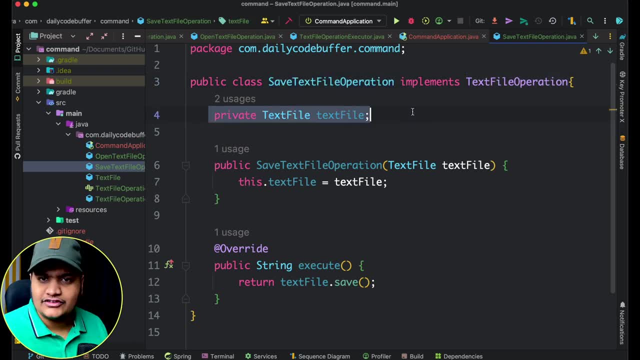 the interface here. This also have the reference of a text file. Okay, This text file is a receiver. We will go to the text file as well. like what it is, text file. But here you can see that for this cell text file we have a constructor and the method implemented. 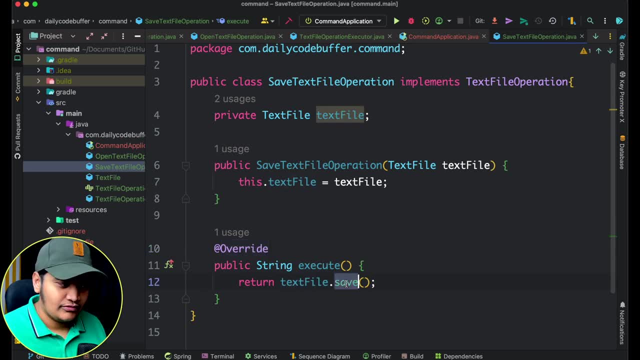 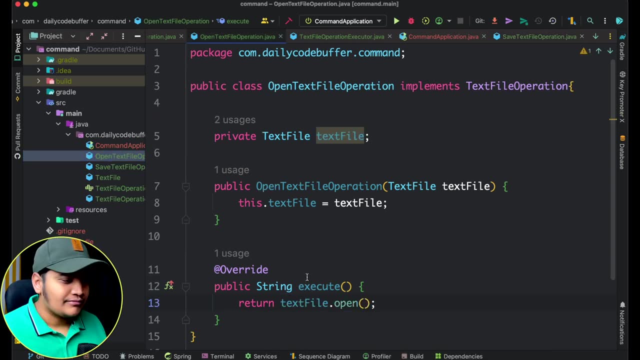 Okay, What we are implementing? we are implementing text filesave. Okay, Here as well, we can do the same thing. We can do text fileopen. Okay. Now, all this method we have placed in the receiver itself. So if we go to the receiver, that is the receiver. 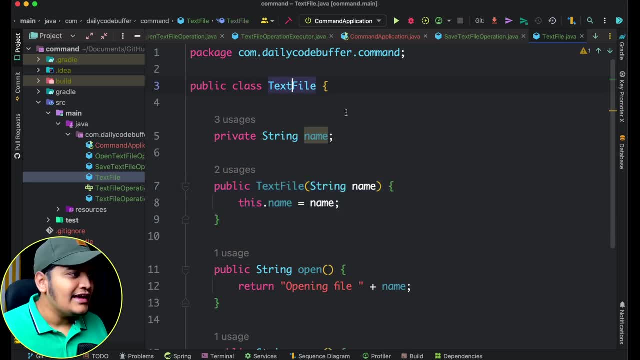 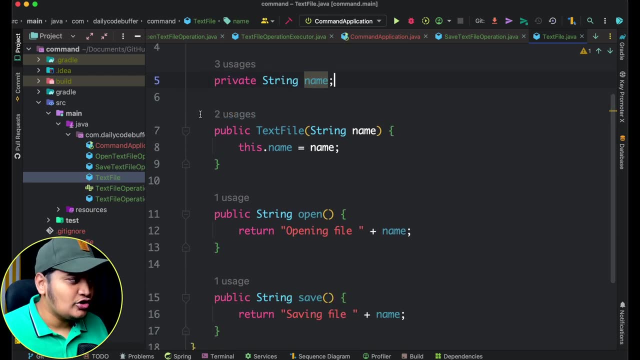 That is the text file. Okay, Here you can see that I've just created simple text file and this text file has some properties. Okay, Suppose it has a name and it has the different methods. This is just a constructor to pass on the name, but it has method. that is the. 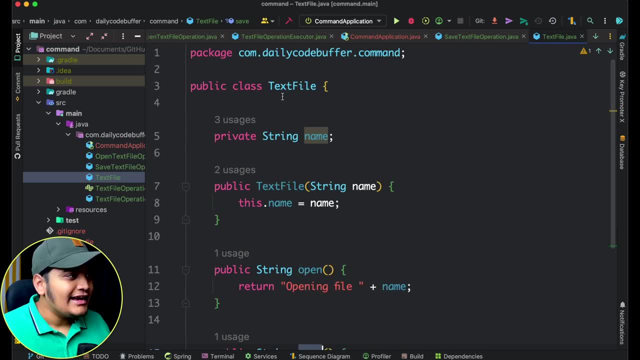 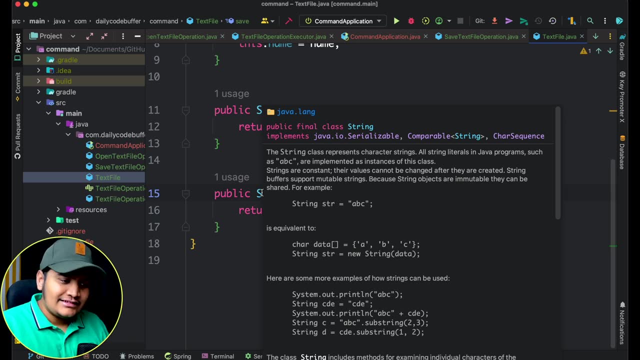 open method and a save method. Okay, So you can see that receiver is something that will actually execute the commands. Okay, So suppose I want to open a file. There is a command I created And with that command I will pass on the receiver and I will call the receivers. 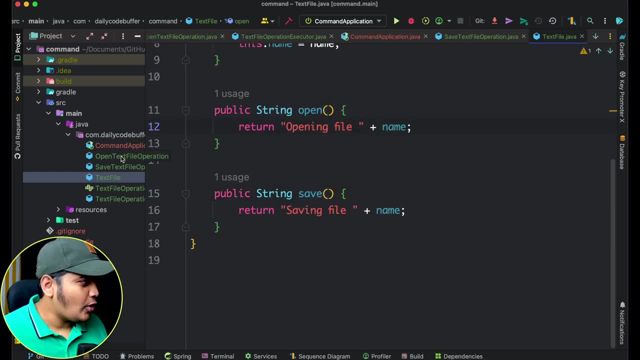 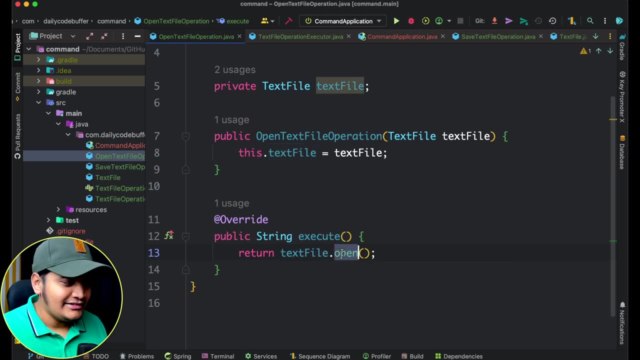 open method. Okay, So here I did the same thing in the open text file command. Okay, I call the execute method And for the receivers class I call this receivers method. That is the open method of a receiver. So that's the same thing over here that I call this open method. 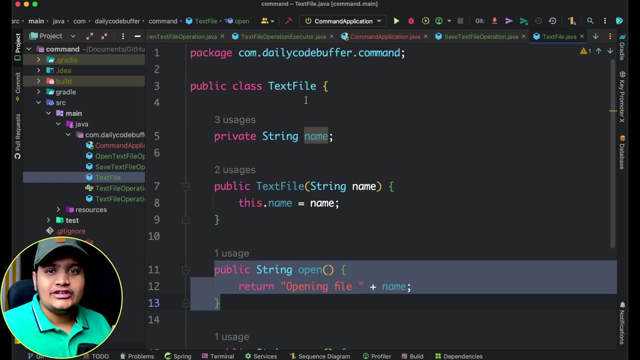 of a text file because I want to open the text file. So these two components we gone through, that is, the command itself and the receiver itself. So that's the relationship between the command and the receiver. Now let's talk about the invoker. So here you. 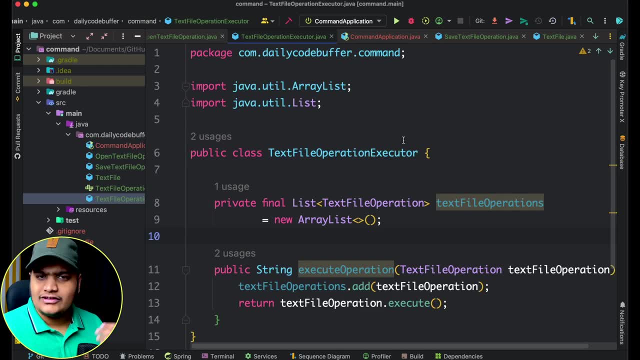 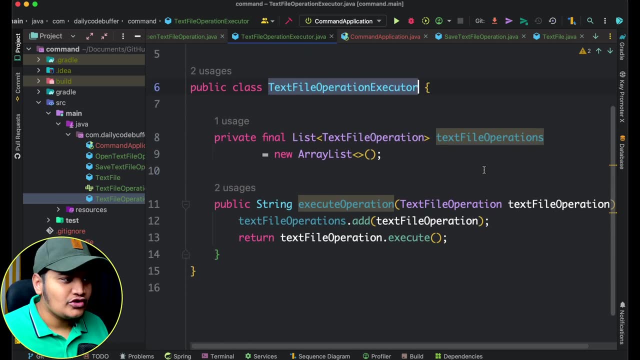 can see that I have created one executor- Okay, You can call it executor or invoker- which will actually invoke the command design pattern. So here you can see that I've just created the class over here and this class have the list of commands to be executed. Okay, Text file- operation. 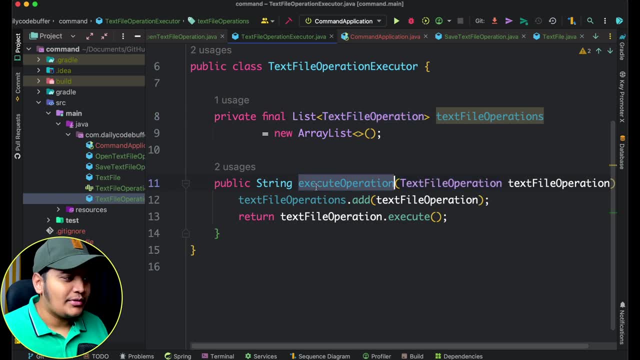 are the list of commands to be executed, and here execute operation. I have defined one method. This method will take on the command and it will add that command to our command list, Like what are all the commands that we have executed, and it will actually execute. 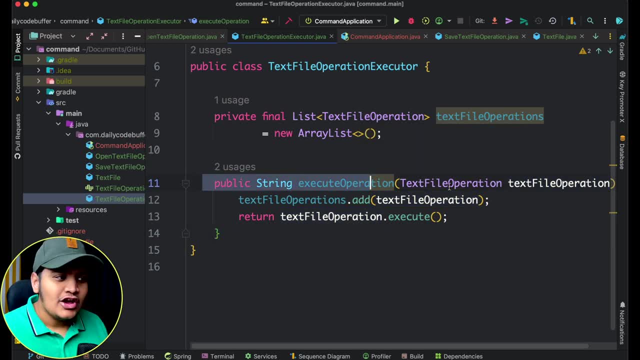 the command. So you can see that this is the method execute operation, which will take the command. It will add the command to our list and it will execute that command. So we will have the entire list as well, Like what all the different commands we have executed. This is helpful. 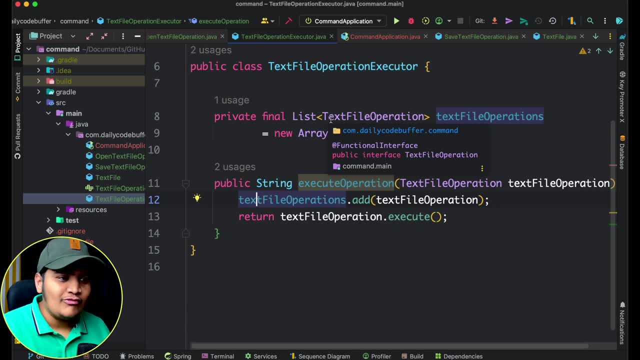 when we want to do undo and redo operations. Okay So this is my invoker. You can have any logic in your invoker. This invoker will be used by the client to execute or to call our command design pattern. Okay, So this is just a simple method which will take the 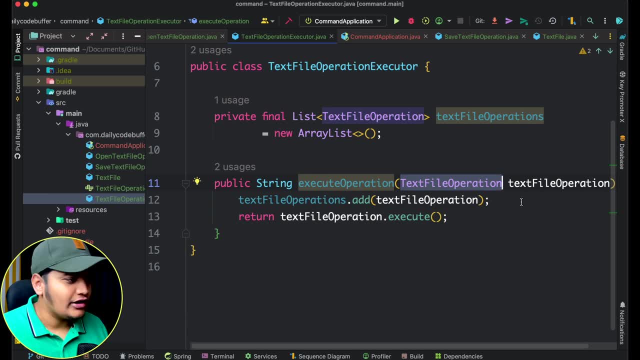 command to execute it. Whatever the command we pass, that will be executed. Okay, So this is just a simple method which will take the command to execute it. Whatever the command we pass, that will be executed. Now let's go to the client. Our client is the command. 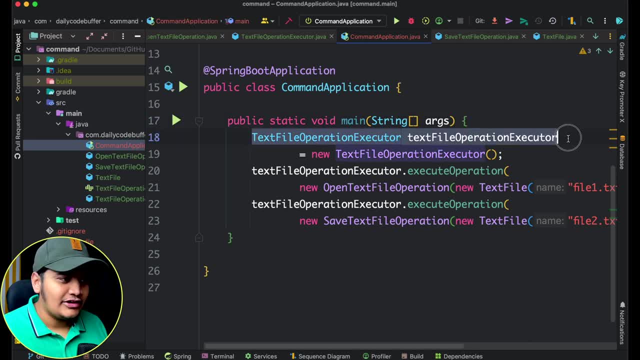 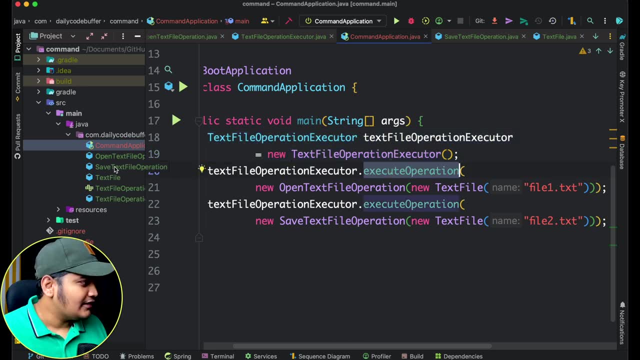 application. Okay, Here you can see that this is the executor that we have created object and within this executor, you can see that in the execute operation- Okay, We have your right execute operation. Let me go back: Execute operation method. is that right in that it? 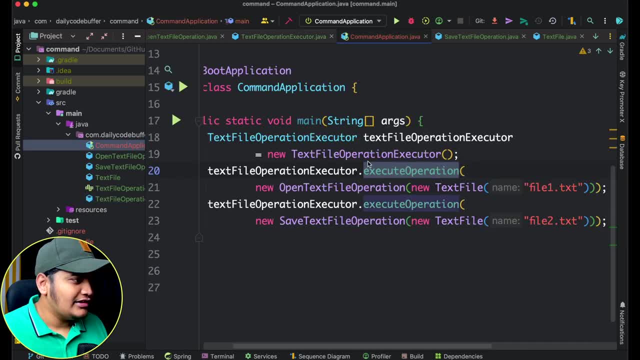 is taking the command itself. So here we are passing within the first executor, means within the first method. what we are passing is we are passing open command, That is, the open text file command. within that I'm passing a new text file and the name of the file.